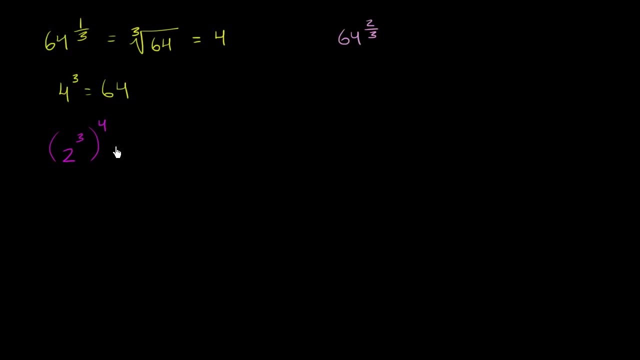 And then I were to raise that to say the fourth power. this is going to be the same thing as raising it to the 2 to the 3 times 4 power or 2 to the 12th power, which you could also write as raising it to the fourth power. 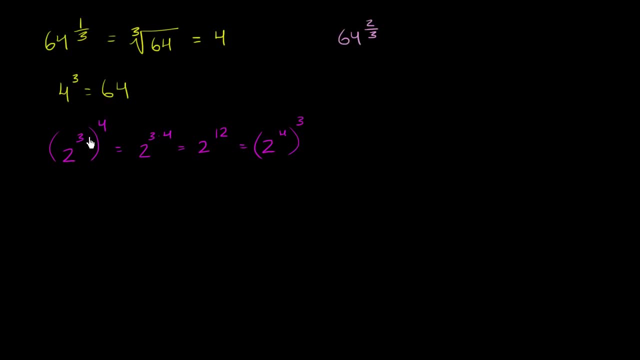 and then the third power. All this is saying is, if I raise something to a power and then raise that whole thing to a power, it's the same thing as multiplying the two exponents. This is the same thing as 2 to the 12th. 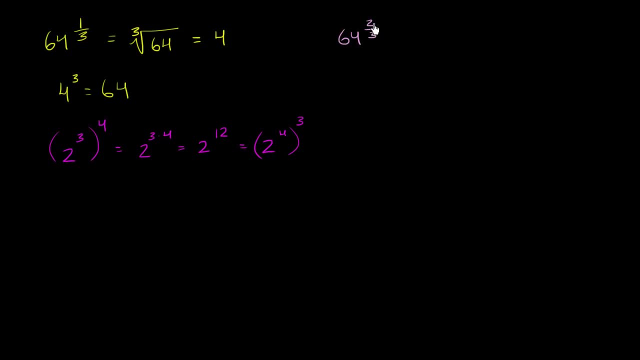 So we could use that property here to say, well, 2 thirds is the same thing as 1 third, 1 third times 2.. So we could go in the other direction. We could say, hey, look well this. 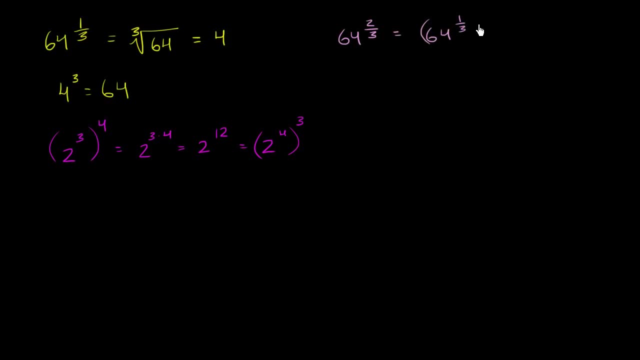 is going to be the same thing as 64 to the 1 third power and then that thing squared. Notice I'm raising something to a power and then raising that to a power. If I were to multiply these two things, I would get 64 to the 2 thirds power. 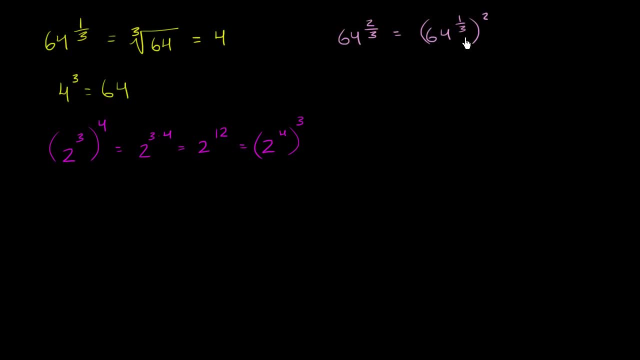 Now, why did I do this? Well, we already know what 64 to the 1 third power is. We just calculated it. That's equal to 4.. So we could say that this is equal to, and I'll write in that same yellow color: 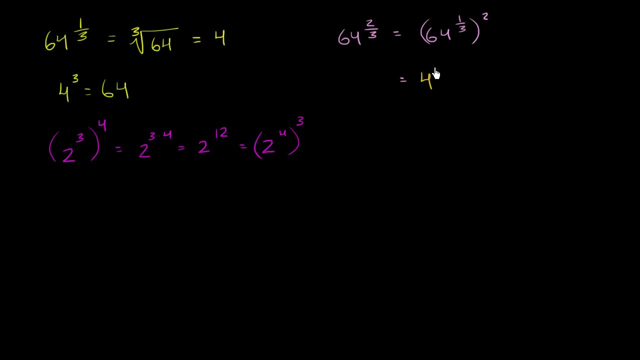 this is equal to 4 squared, which is equal to 16.. So 64 to the 2 thirds power is equal to 16.. The way I think of it, let me find the cube root of 64, which is 4, and then let me square it. 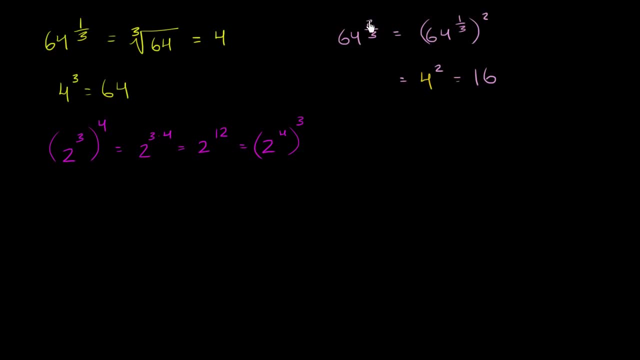 And that is going to get me to 16.. Now I'll give you an even hairier problem, and I encourage you to try this one on your own before I work through it. So we're going to work with 8.. 8 over 27.. 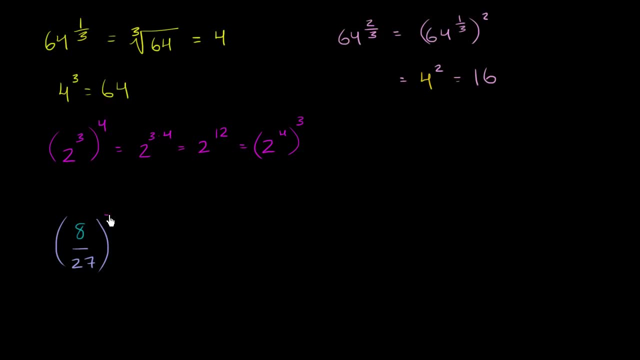 And we're going to raise this thing to the negative- and I'll try to color code it: negative: 2 over 3 power to the negative 2 thirds power. I encourage you to pause this and try this on your own. Well, the first thing I do whenever 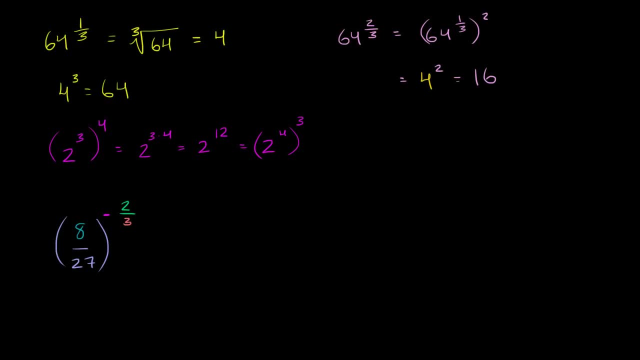 I see a negative exponent is to say: well, how can I get rid of that negative exponent? And I just remind myself: well, the negative exponent really just says: take the reciprocal, Take the reciprocal of this to the positive exponent. So this is going to be equal to. the reciprocal of this is 27.. 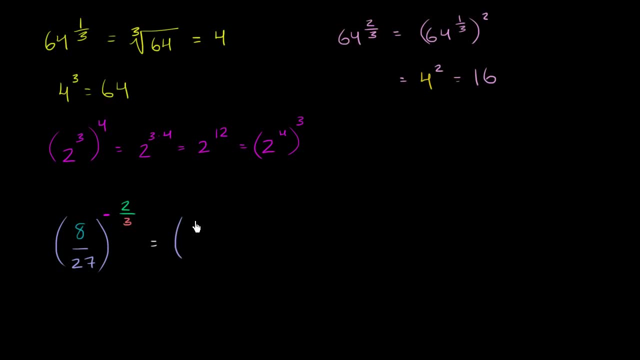 I'm using a different color. Let me use that light mauve color. So this is going to be equal to 27 over 8.. I just took the reciprocal of this right over here. It's equal to 27 over 8, to the positive 2 thirds power. 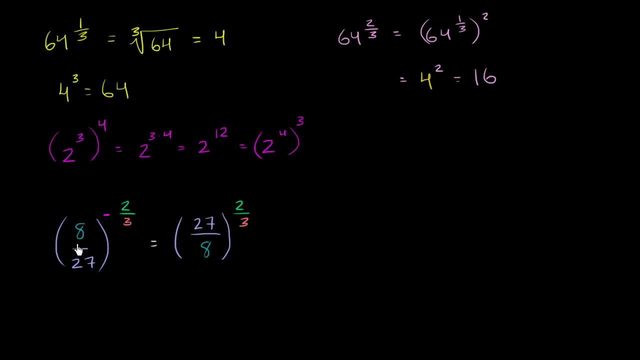 So notice, all I did: got rid of the exponent and took the reciprocal of the base right over here: 8 over 27 is the base, Negative 2 thirds is the exponent. Now how can we handle this? Well, we've already seen that if I 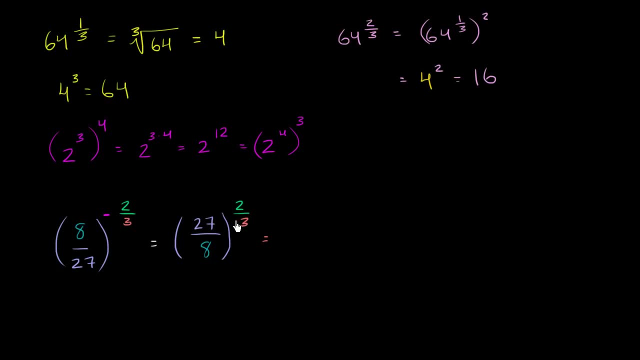 have a numerator sum power over denominator sum power, and this is another very powerful exponent property. this is going to be the exact same thing as raising 27 to the 2 thirds power Over 8 to the 2 thirds power. This is another very powerful exponent property. 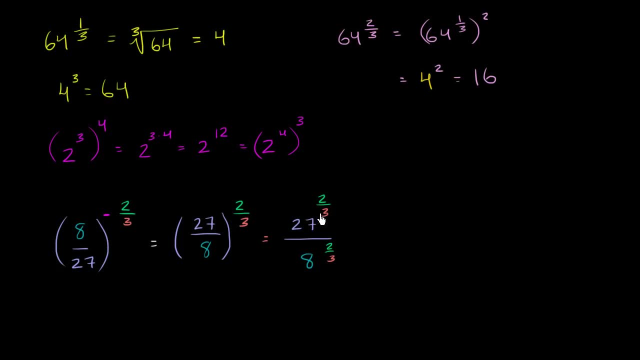 Notice, if I have something divided by something and I'm raising the whole thing to a power, I can essentially raise the numerator of that power over the denominator raised to that power. Now let's think about what this is. Well, just like we saw before this: 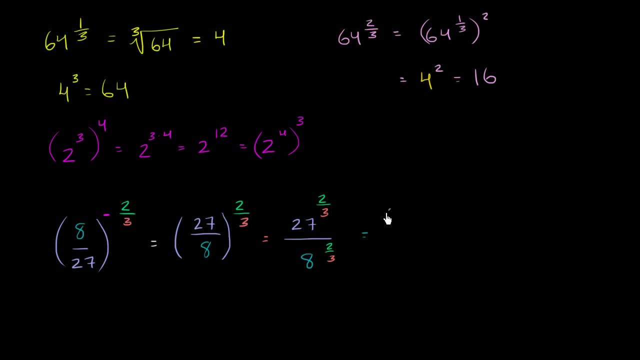 is going to be the same thing as 27 to the 1 third power, 27 to the 1 third power, And then that squared because 1 third times 2 is 2 thirds. So I'm going to raise 27 to the 1 third power. 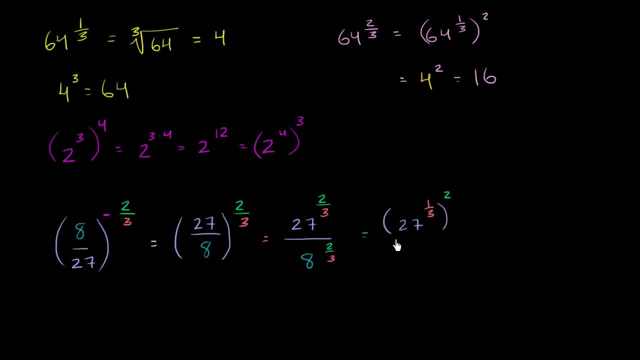 and then square whatever that is And that is going to be over. all this color coding is making this switch a lot of colors. This is going to be over 8 to the 1 third power And then that's going to be raised to the second power. 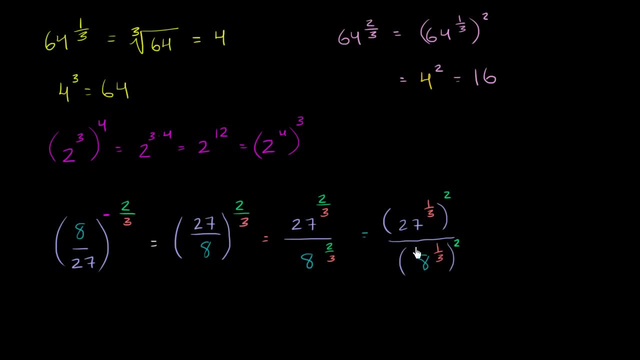 Same thing we're doing in the denominator: We raise 8 to the 1 third And then square that. So what's this going to be? Well, 27 to the 1 third, power is the cube root of 27.. It's some number. 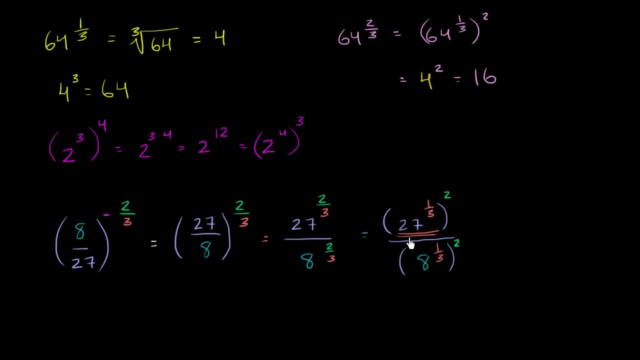 That number times that same number, times that same number, is going to be equal to 27.. Well, it might jump out at you already that 3 to the third is equal to 27,, or that 27 to the 1 third is equal to 3.. 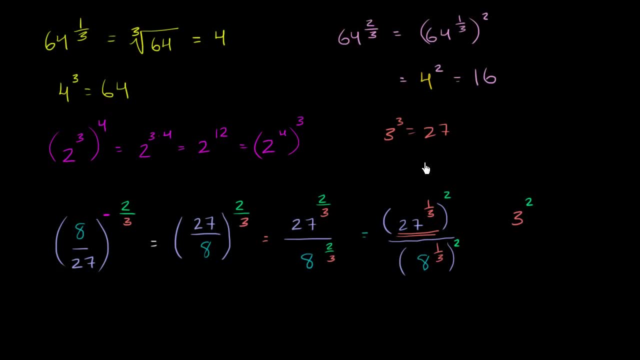 So the numerator, we're going to end up with 3 squared, And then in the denominator, we are going to end up with: well, what's 8 to the 1? third power? Well, 2 times 2 times 2 is 8.. 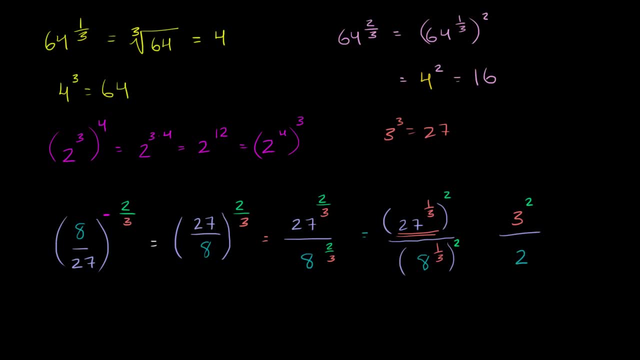 So this is 8 to the 1, third is 2.. And then we are going to: and then let me do that same orange color: 8 to the 1, third is 2.. And then we're going to square that. 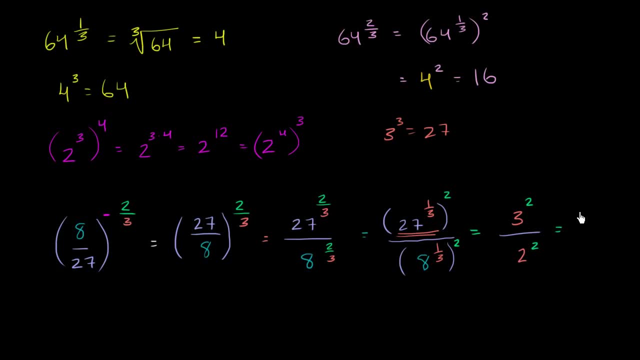 So this is going to simplify to 3 squared over 2 squared, which is just going to be equal to 9 over 4.. So if you just break it down step by step, it actually is not too daunting.